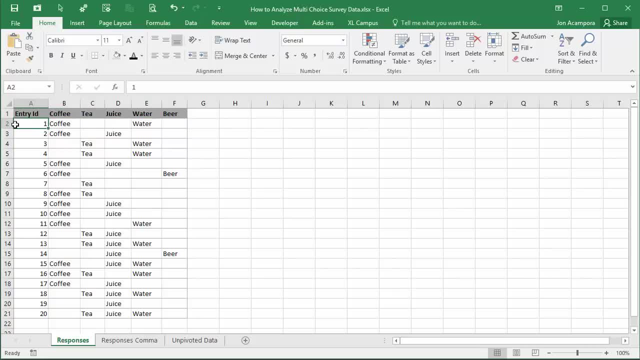 the user can choose, and then each row in the data down below contains a response from one person. So this person here chose both coffee and water as their responses, and we had 20 total responses for the survey. So in this video here, we're going to look at how to transform this data with Power. 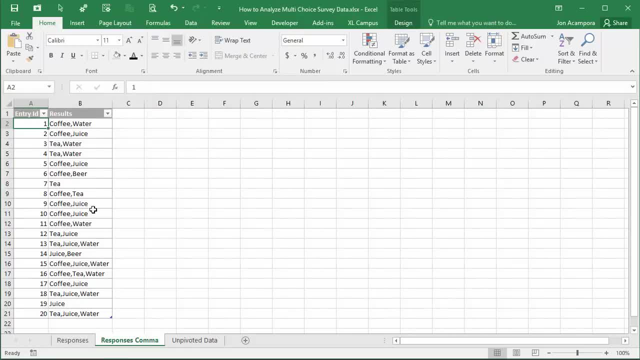 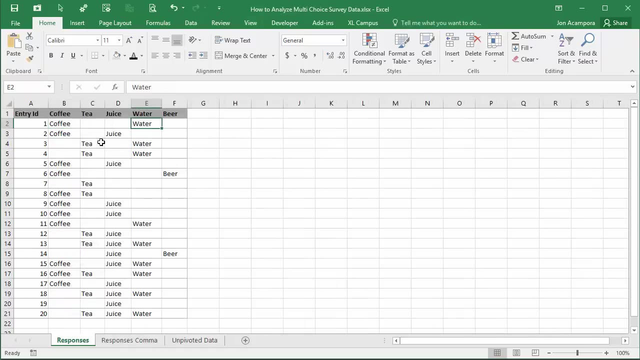 Query. In the next video we'll look at this format, which is more of comma separated values, where we have one column of results with comma separated values. So we'll look at how to transform that with Power Query in the next video. So in this video here we basically want to take this format. 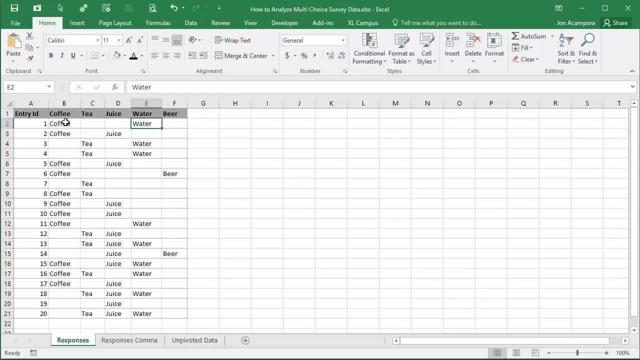 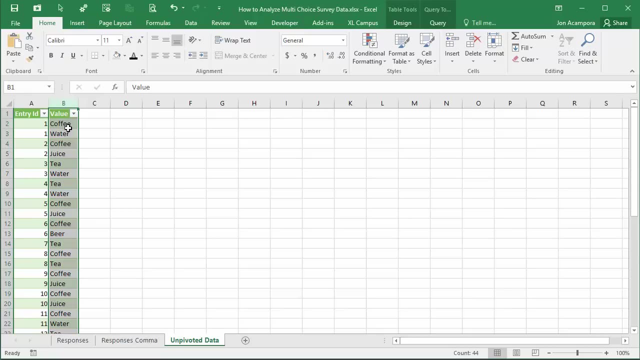 this data that's in this layout and use the unpivot feature in Power Query to get it into a layout that's more user-friendly for a pivot table. And that layout looks like this here, where we have one column of values here, which would be the results, and then multiple rows for each entry. 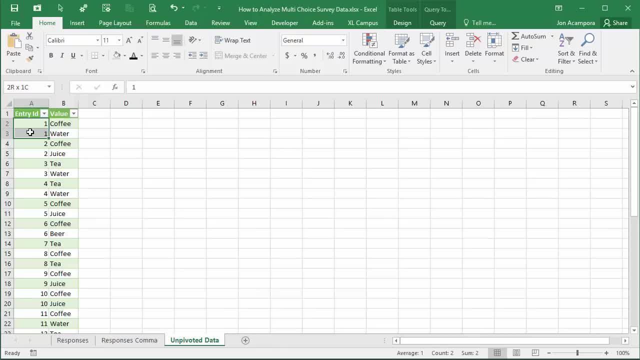 So we can see here that this we'd have two rows for entry number one. this would be for the results, for one person and then both of their rows would be for one person. So we can see here that this would be for one person and then both of their rows would be for one person and then both of their. 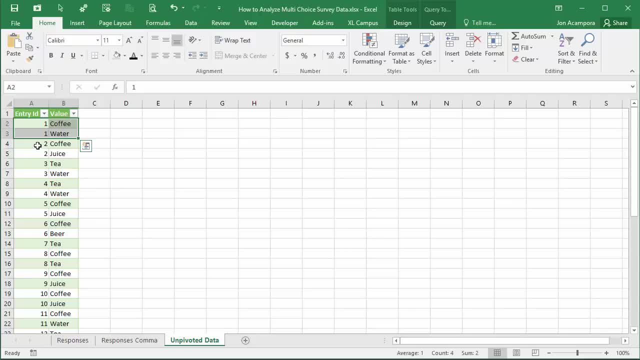 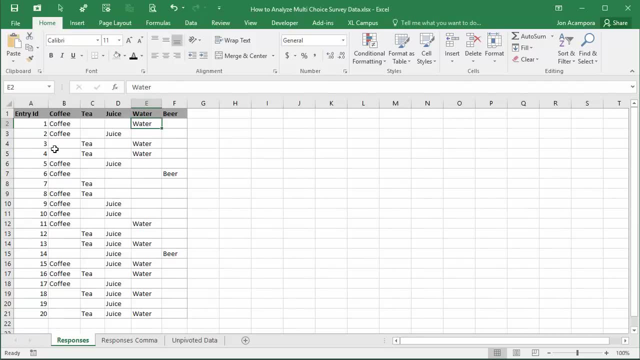 results listed here in the same column and so on. it goes down for the rest of the people that took the survey. So we're basically going to transform this data using Power Query to get it into this type of layout here that we can use for a pivot table. So to do that, the first thing we need to do- 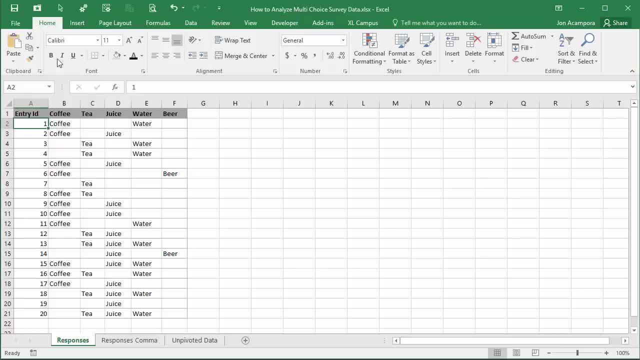 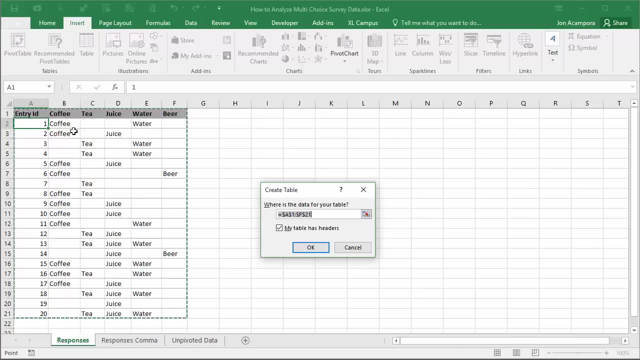 is: convert this to an Excel table. You can hit ctrl t on the keyboard or go to the insert tab on the ribbon and choose table. You'll just want to have any cells selected inside the range first. that'll bring up the create table. prompt should automatically select your range for you and then. 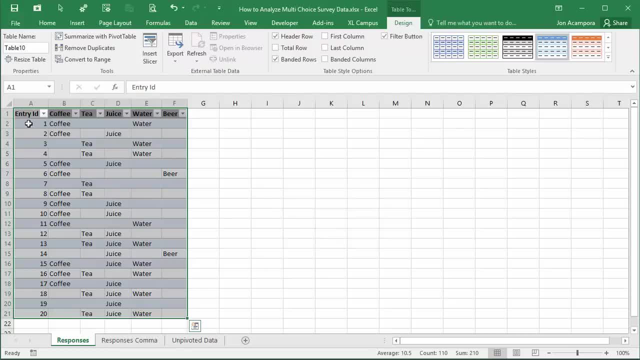 click ok. So now we have an Excel table here. you can go and change the formatting of this if you like, but basically now we're going to use Power Query to transform this. So I'm going to the data tab on the ribbon. I'm using Excel 2016 for this video. Power Query is now in the get and transform. 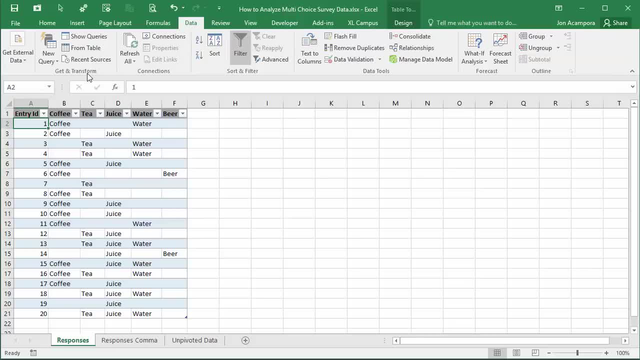 section of the data tab. If you're using Excel 2010 or 2013 for Windows, then you'll install Power Query and it'll be in a separate tab. in the ribbon up here It'll say Power Query, and I have other articles and videos that go over that in more detail. I'll put the links to those below So we're 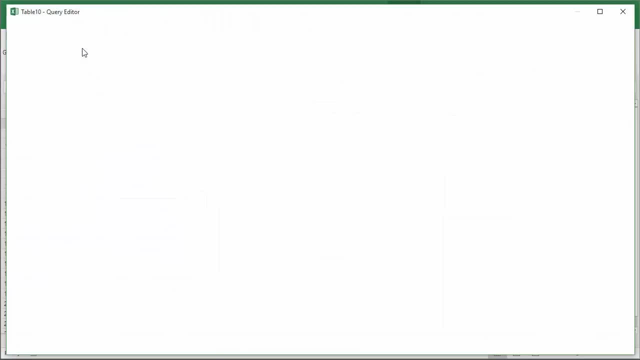 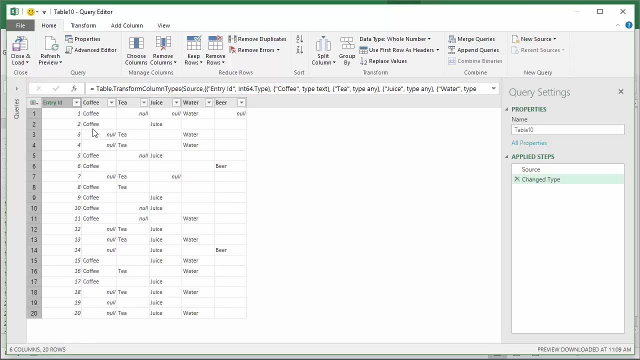 basically just going to choose the from table button here and click the from table button. That'll bring up the Power Query editor window and now we just need to transform this data. So here I have a preview down here of my data. I'm going to go to the transform tab up here on the ribbon and use the 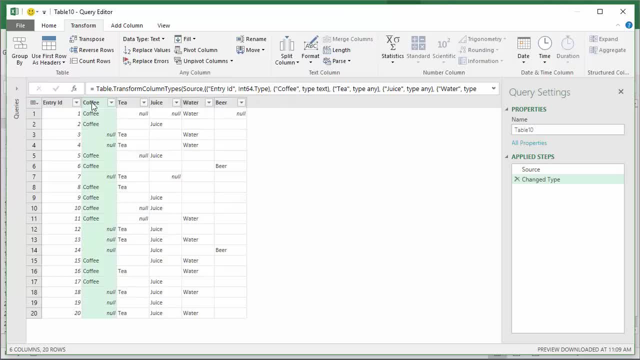 pivot columns feature. So first thing I'm going to do is just select the columns I want to unpivot. I'm going to left click coffee, then I'm going to hold down the shift key on the keyboard and select beer, and then I'm going to click the unpivot columns button here and that's basically now made that. 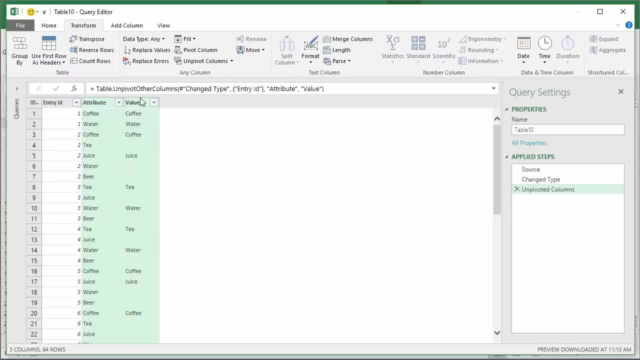 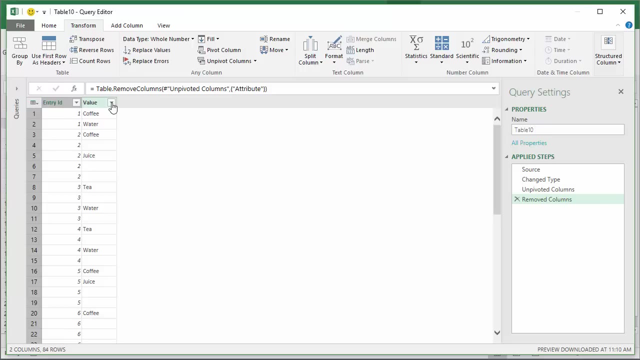 transformation very quickly for me. So now I have one column of values here. These are all the responses from the surveys, and then the attribute column is basically all the column headers. We actually don't need this column, So I'm going to right click and remove it, And then the other thing I want to do is I want to remove all. 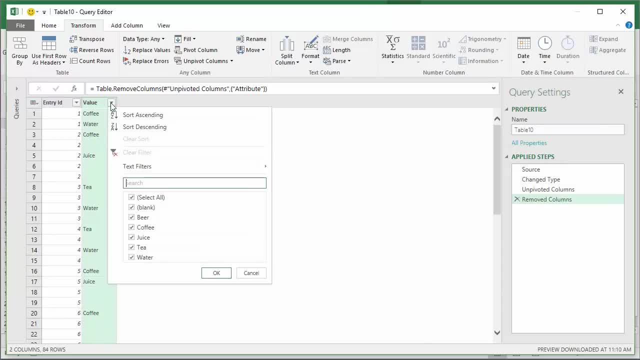 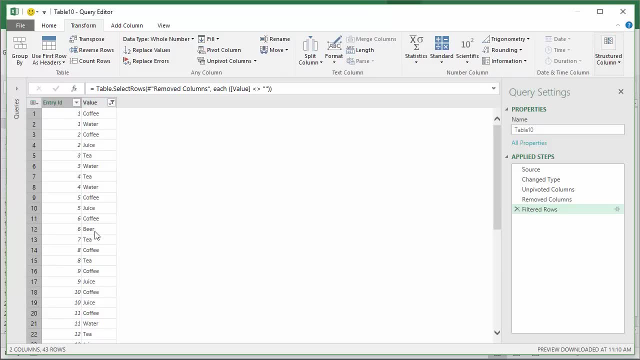 of these blank cells here. I don't need all these blanks. I'm just going to click the filter button here and uncheck blank and click OK and that'll remove all the blanks. So now I have a nice clean table that I can use as a source of a pivot table. So I'm going to go to the home tab on the ribbon here and click the close. 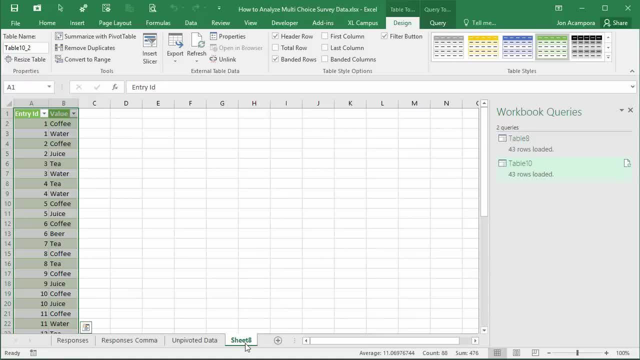 and load button and that'll basically create a new sheet And then I'm going to go to the workbook with the output of my query. So again, here's my table that I can now use as a source of a pivot table. So this is great. It's very easy to work with, to use the pivot table. and then we're going to 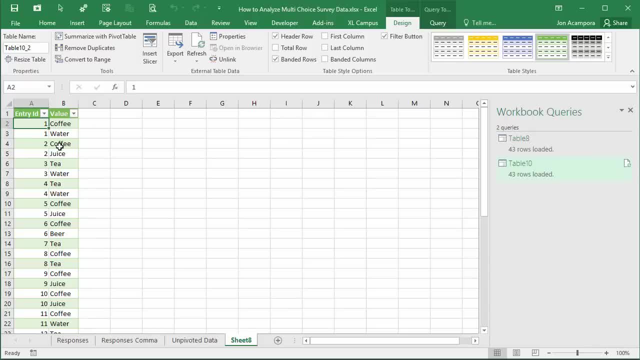 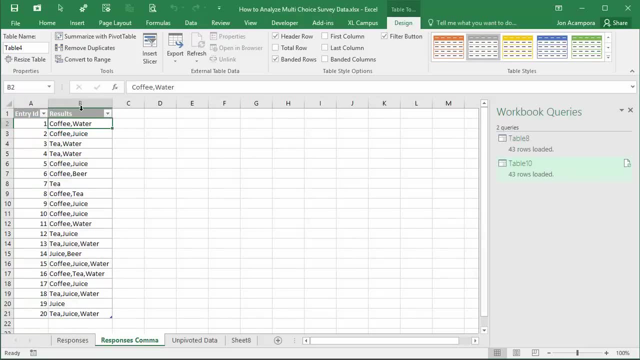 summarize this and analyze this data. So in the next video I'm going to show that exact same process, but with this list of results. here, that's basically one column of comma separated values, And then in the third video we'll look into how to summarize.